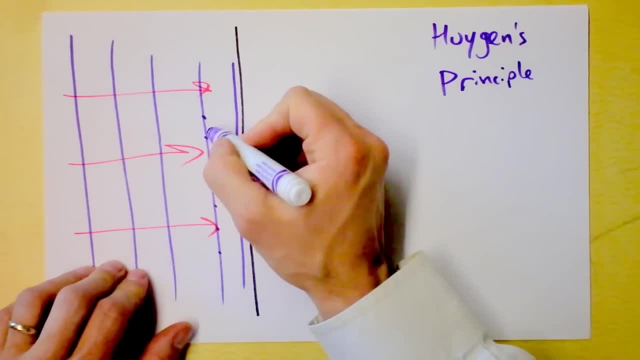 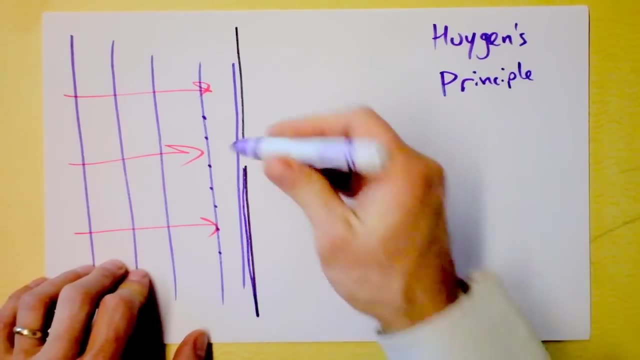 So every point on this wave front here is creating a new spherical wave front. So what's happening as we reach this barrier is that all of the wave here is being blocked, and all of the wave here is being blocked, so we're able to actually see Hohen's principle at work. 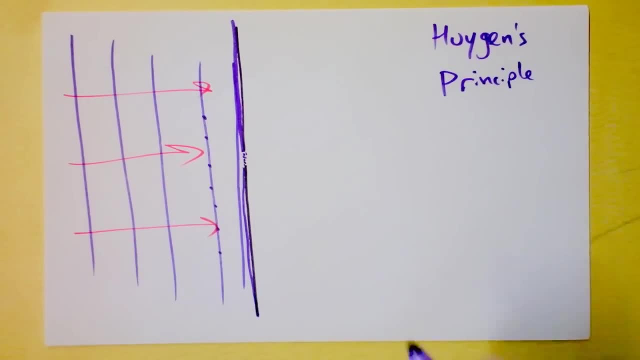 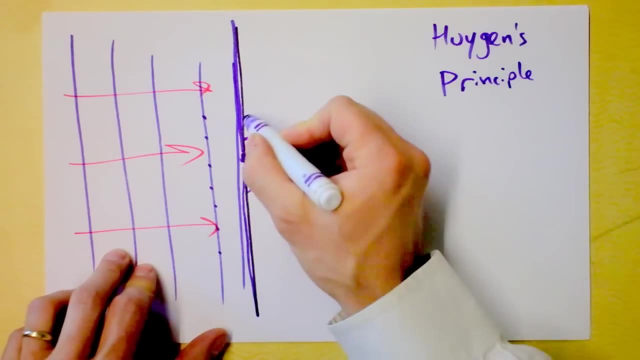 These locations- Hohen's principle H-U-Y-G-E-N, These locations H-U-Y-G-E-N, These locations right here are very close to each other and they become locations from which a new wave springs, and that's why sound can bend around a corner. 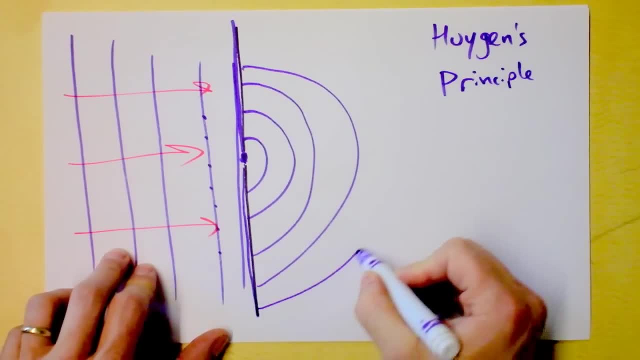 Perhaps you didn't believe that sound can bend around a corner. Perhaps you never believed that sound was a wave. Well, let me prove it to you. I'm going to go around the corner. I'm literally going to be on the opposite side of this door, and you can still hear me. 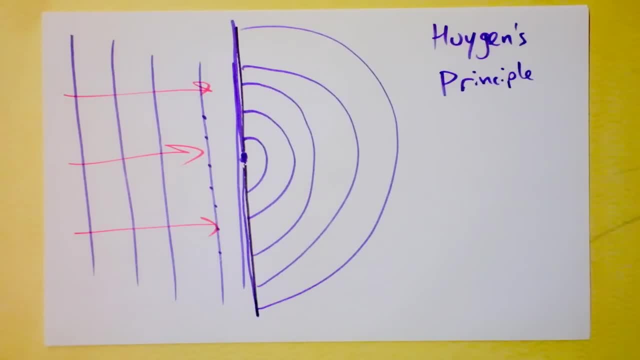 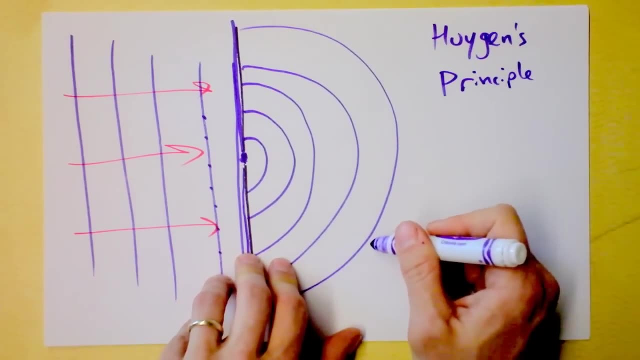 Yeah, I'm quieter, but it's not reflection that you're hearing. Primarily you're hearing the sound bend around. If we were to set this up really clever-like, I could make you another little barrier over here. Let's say I make a barrier in this big old room. 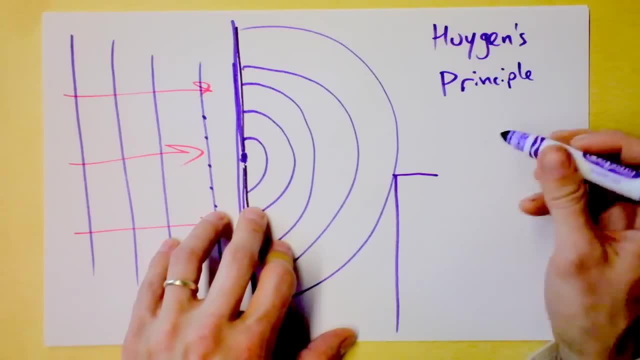 I make a barrier right here And what's gonna happen is maybe I should angle a little bit more gently. No, it's cool. Every point on here I'm gonna have this coming in like this and it comes in like this: 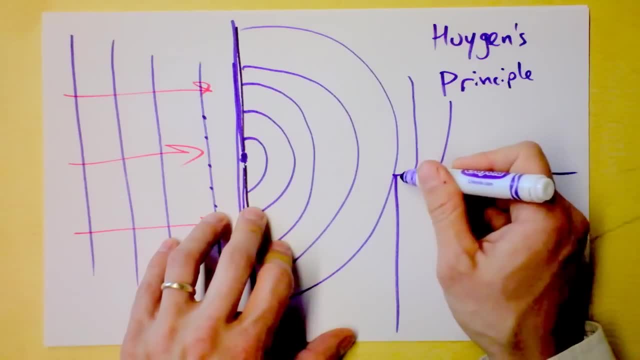 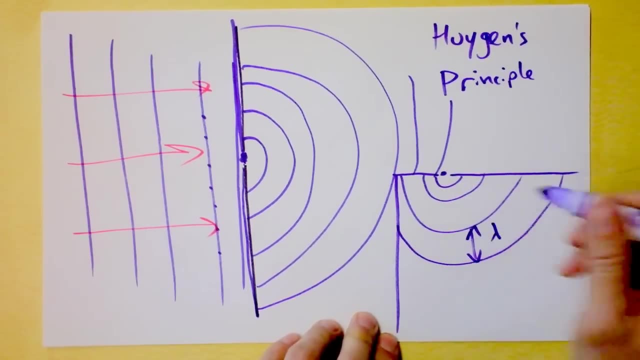 and this location right here becomes a new wave front, and now I've got waves that come out like this: They're supposed to have the same wavelength all the time if I'm in the same medium, so this should be the wavelength and it should be equal to this wavelength that's over here. 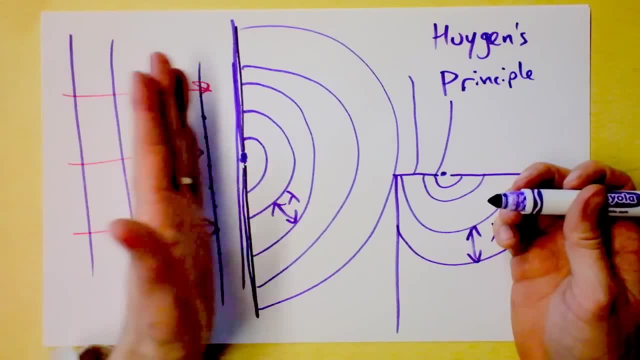 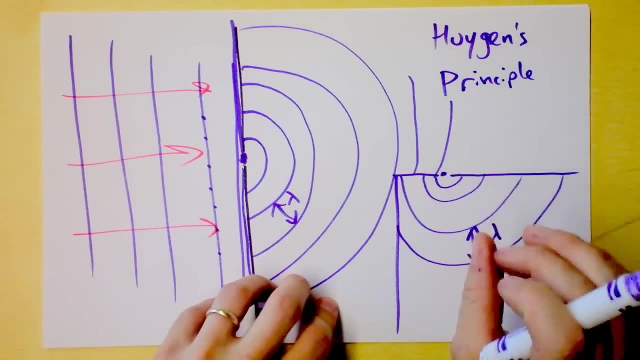 But notice that now I've got waves that are going back when my original waves were going this direction. I hope that doesn't bother you. It's a little bit weird, but Herman's Principle is really, really weird when you try to apply it to a wave. 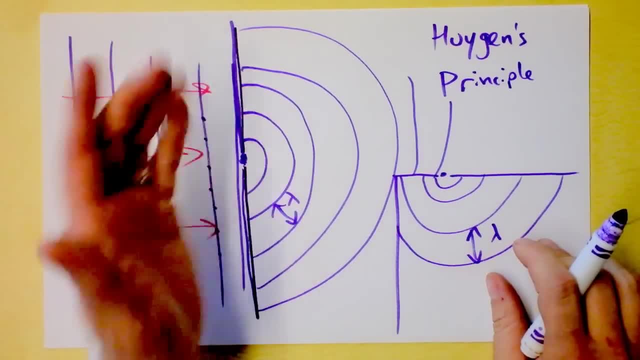 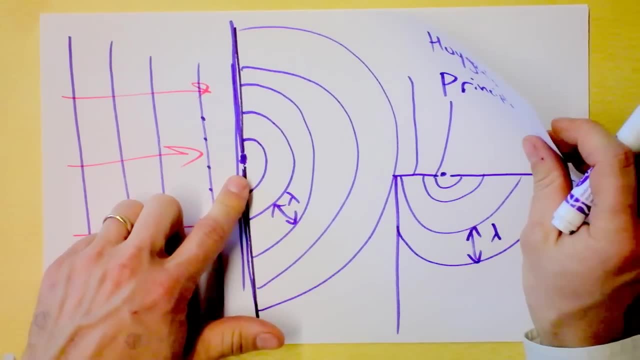 that's just a plain wave like this just moving in And let's see if we can make some sense out of that. But here's Herman's Principle at an interface. Wait, this means some really cool things for us. This means some 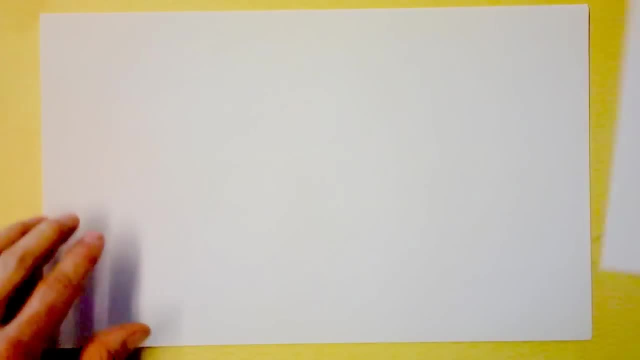 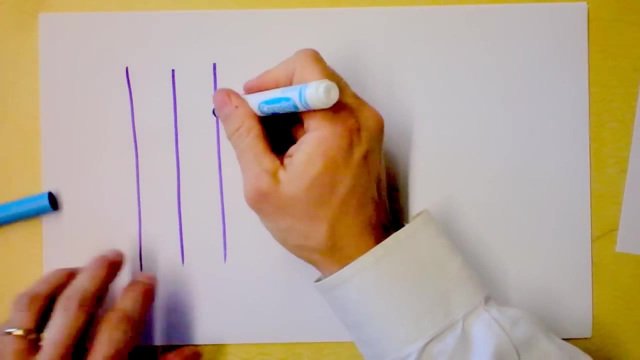 really cool things. Well, we'll look at that in just a moment. First, we have to figure out how a plain wave can be represented by Herman's Principle. I'm gonna study three locations on this plain wave. Nah four, This one, this one, this one and this one. 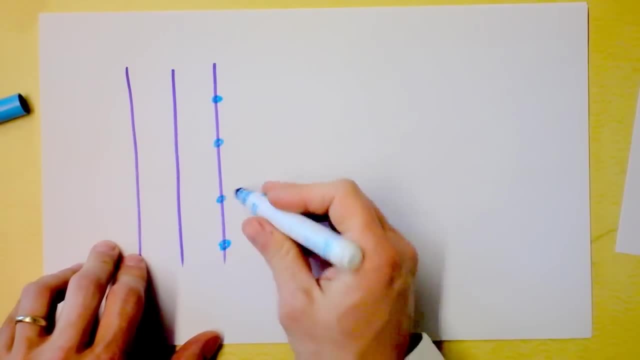 And if I treat each of these as being a source of new waves, then I'll say that, well, here's the wavelength right. So I'm gonna say that, right here it will make a new wave, right, and right here this one will make a new wave. 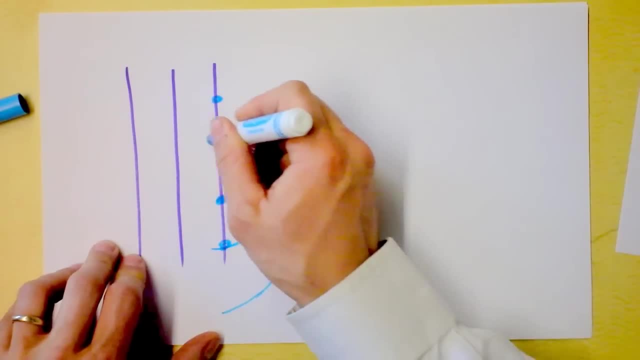 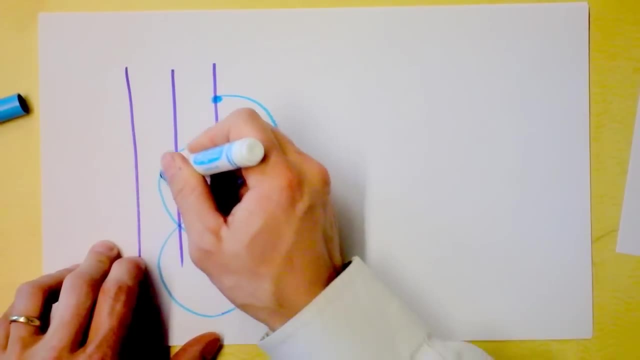 that's like: hang on just a second like that, right going out like that. This one makes a new wave that's going out like that. This one makes a new wave. sorry, this one makes a new wave that's going out like that. 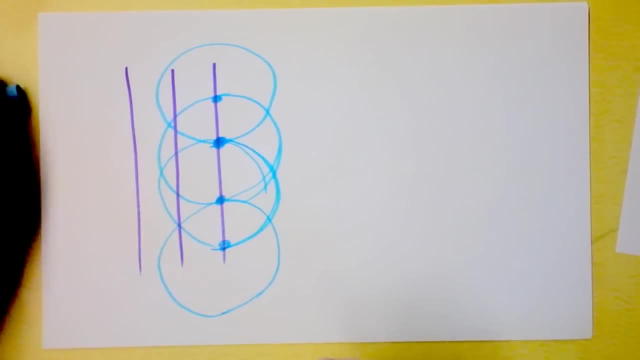 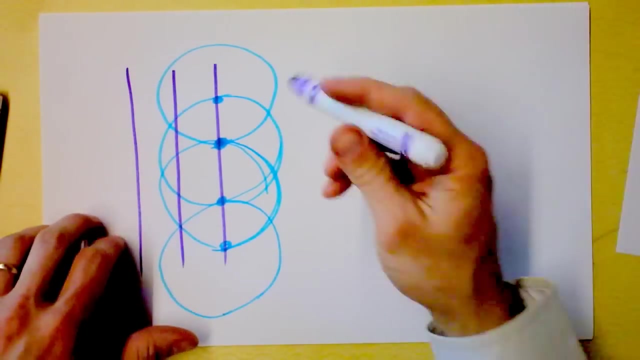 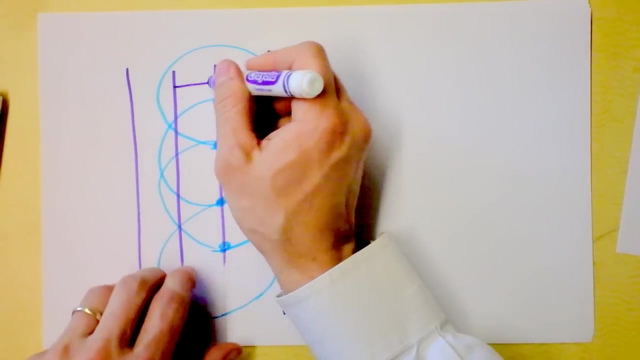 And this one makes a new wave that's going out like that. Now, the interesting thing about this new wave that's been formed by each of these four points here is that we're going to get constructive interference right here at the front, And the cool thing is that a moment later, this wave became that wave, and 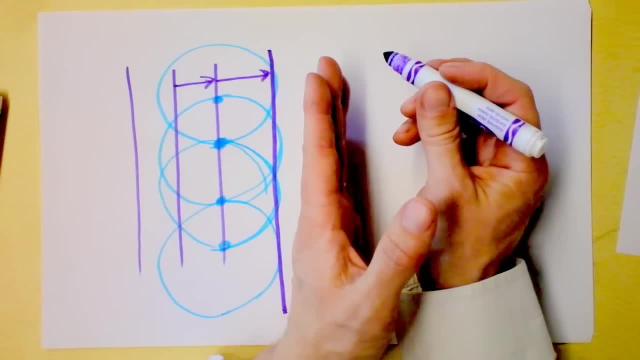 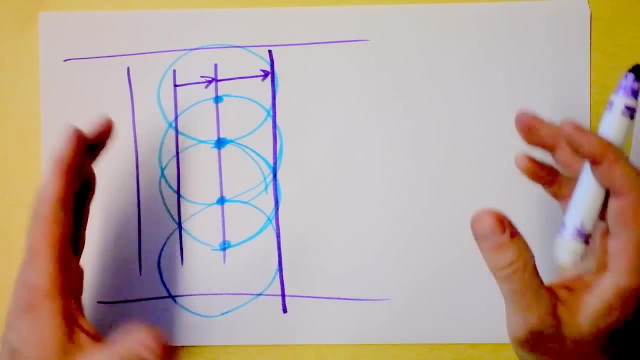 this wave becomes that wave, and so that's the progression of the wave. If we've got a flat wall here and a flat wall here, that wave's just gonna move right on through, And principle is simply a statement that plane waves can move unimpeded. 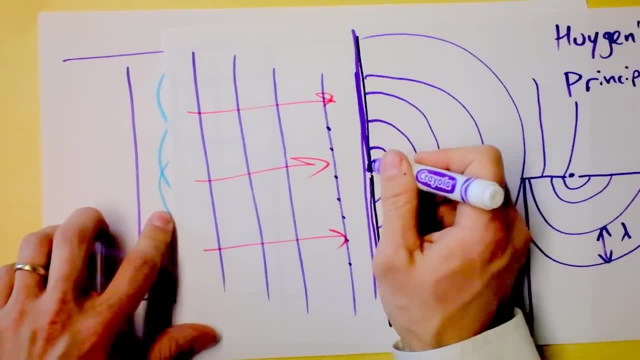 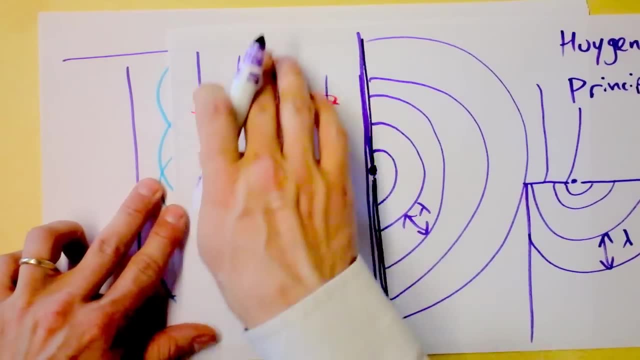 But if you get to a break where only one of these new wave fronts, these new spherical wave fronts, is able to get through, it's then that you see that a plane wave is actually made up of an infinite superposition of spherical waves. Whoa. 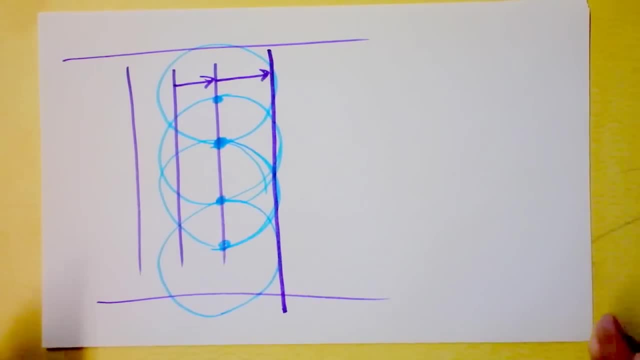 A plane wave is an infinite superposition of spherical waves. That's pretty cool. The next thing we need to do with Herron's principle is give you a barrier that has two gaps in it, And then we're going to have ourselves a very interesting experience. This was Young's idea. It was 1804.. Lewis and Clark were out to explore the. what was he gonna do? Was it 1801 or 1804? I don't know. I'm getting some conflicting opinions, But anyway, we were certainly about to buy the Louisiana territory, or? 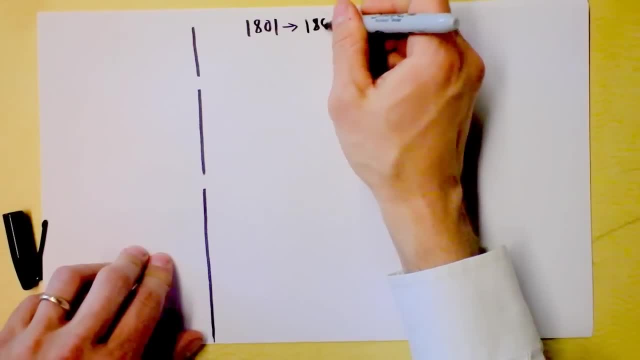 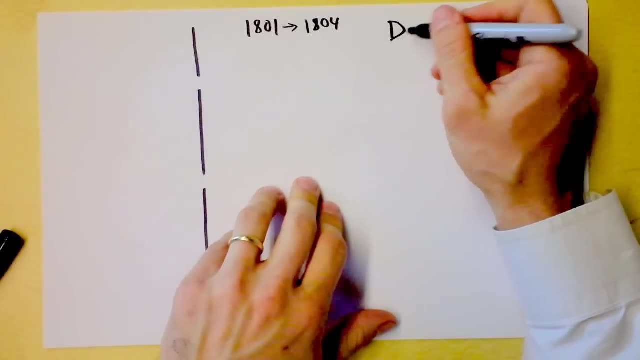 had just bought the Louisiana territory or something in the United States And sometime around there, this fella named Young over in England had a great idea. He was so brilliant, he deciphered. check this out. This guy deciphered the freaking Rosetta Stone. 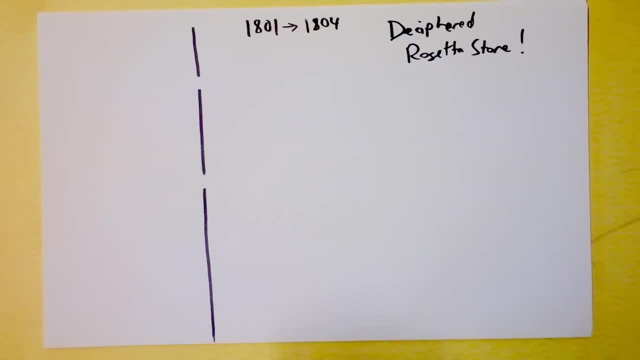 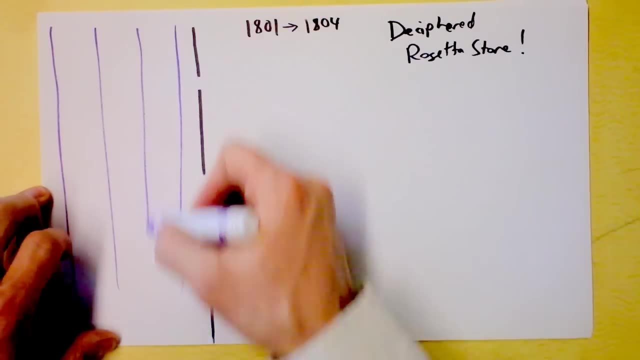 And founded that software company. just kidding, He actually deciphered the actual Rosetta Stone. And if I have waves coming in here, and the waves, well, they're coming from this direction. If waves are coming in here like this, then I'm gonna see Herron's principle right here.